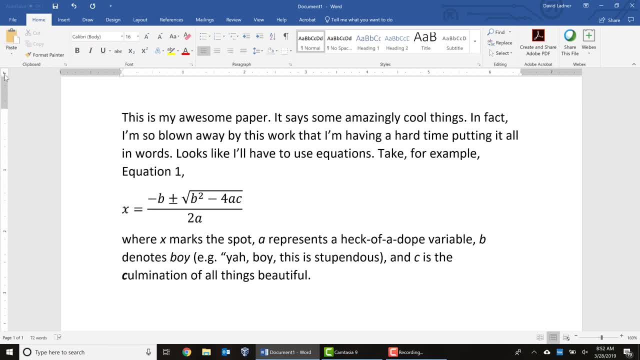 So first thing I want to do is change this tab stop from a left tab to a center tab and I'm going to put that at 3.25, which is the center of this particular document. And then I'm going to do another tab stop on the right, so I clicked this to turn it to a right tab stop and I'll put that over there. 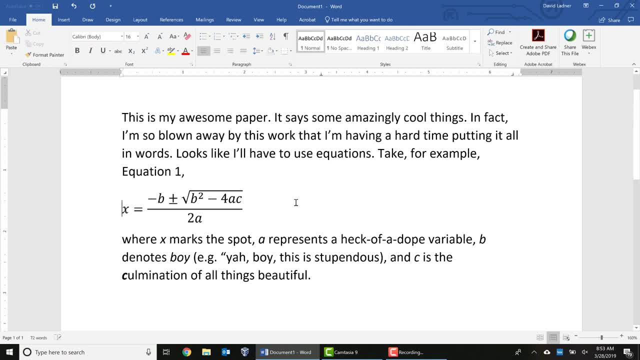 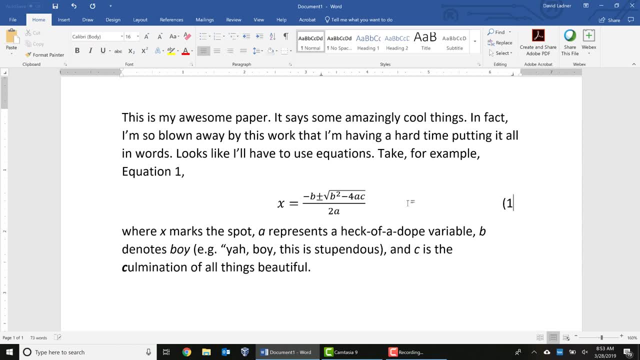 Now I'm ready to go to the beginning of this and press tab that centers the equation. and on the other side of the equation I press tab again and I'll put my number in. And there we go Now. if I want to repeat this for other equations, I'll just copy the whole thing. 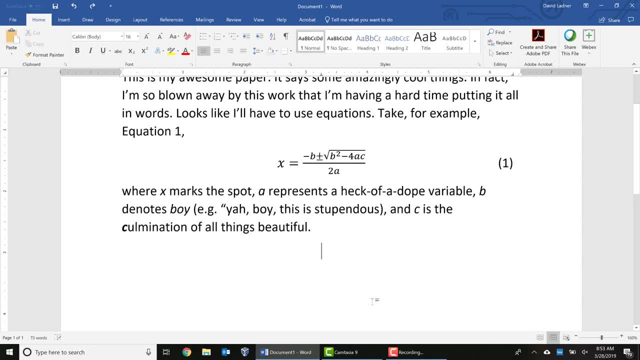 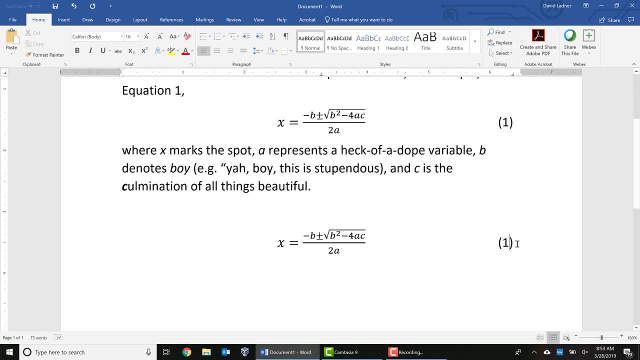 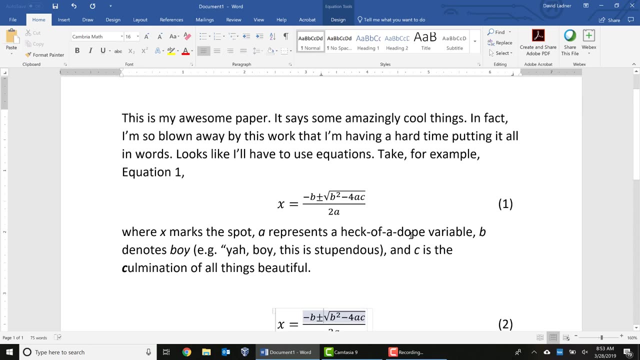 And paste it down here. Oh, that did not work, did it Hit a new line return? and there we go, Paste it down there, and the centering is good and the right numbering is good, and then I can just change the equation. That's really all there is to it as far as lining up equations and their numbers. 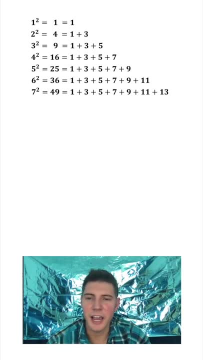 Have you ever looked at all the perfect squares and realized that you just have to add the next odd number to get to the next perfect square? Here it is written out right here, and this is a true pattern. Would you like to know why it is? We start with 1 squared and that's 1.. And then 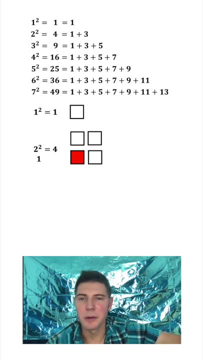 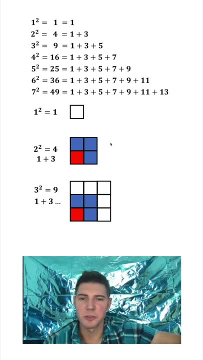 2 squared becomes 4.. But if we break this out, 2 squared is made up of the original 1 plus 3 more, and that's why it's 1 plus 3.. If we look at 3 squared, we have the original 1 plus 3 from the. 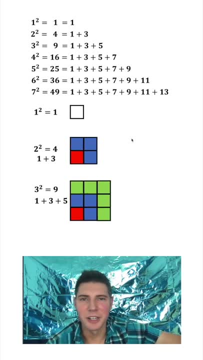 1 before, and we're going to add to it these 5 outside here. That's how we get to the 9.. If we look at, 4 squared equals 16, here's the 1 from before. Then we have these 3,, these 3, and this. 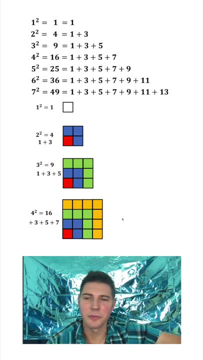 1, which is the 7 that we're adding to the outside of this 1.. And that's how we get: 4 squared equals 16.. So you can see what's causing the pattern. We have these two sides, which is always going to be. 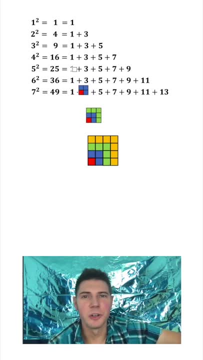 an even number plus 1 more, which makes it an odd number. But we can also show it in the general case. If we do this as n by n, the area would be n squared. Now what is the next one? n plus 1.